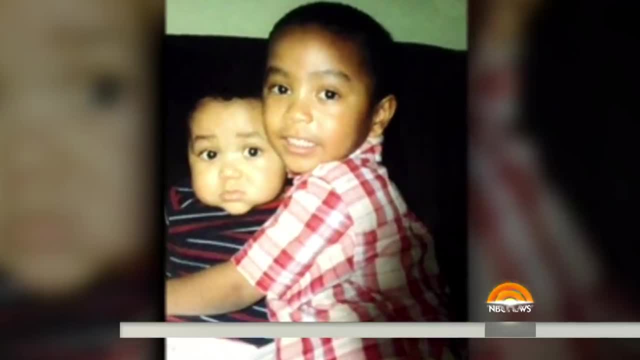 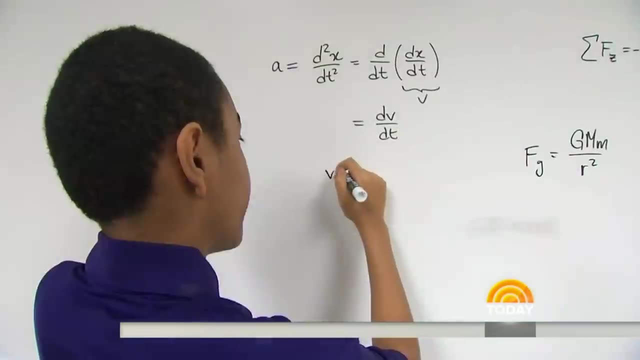 She homeschooled Carson until he was five, when she knew he needed more. So she took me to a public school and they said that I was way too advanced. I ended up going to a high school- private high school- A five-year-old in eighth grade. 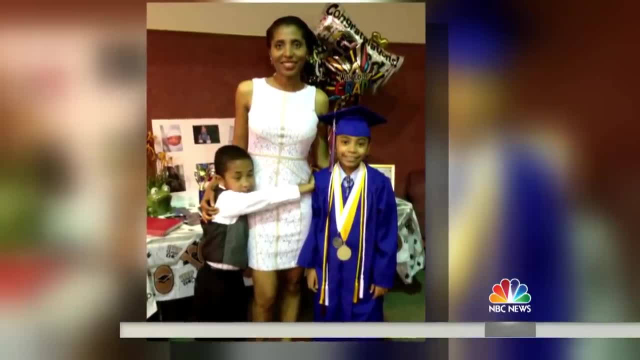 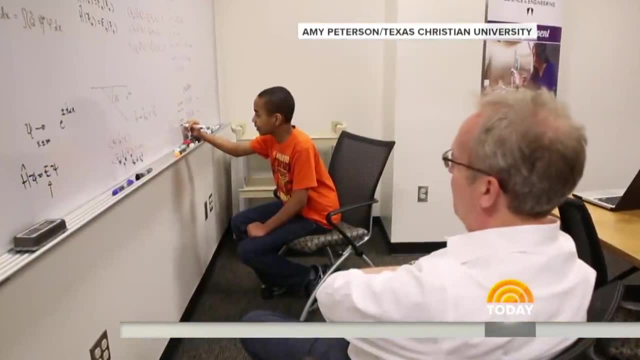 After that, I didn't skip anything and graduated at 10 years old. That 10-year-old boy dove right into physics. when he got to TCU It would become his major, along with a double minor in math and Chinese. Professor Magnus Ritby became a mentor to Carson. 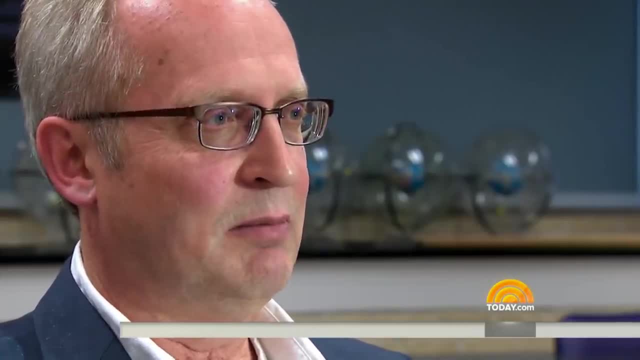 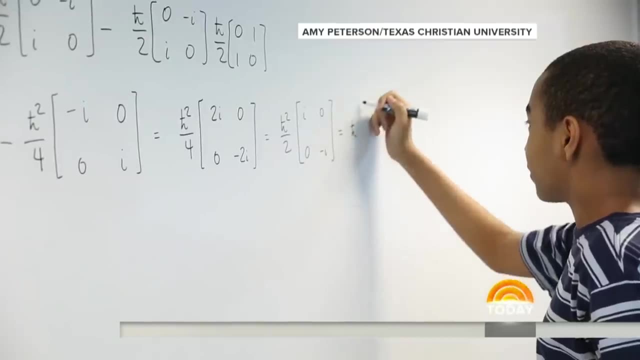 One of the main principles I've always been: Don't give him preferential treatment. Try to really treat him as any other college kid. Of course, Carson really isn't your average college kid. I still play games. I have my little brother, Cannon. 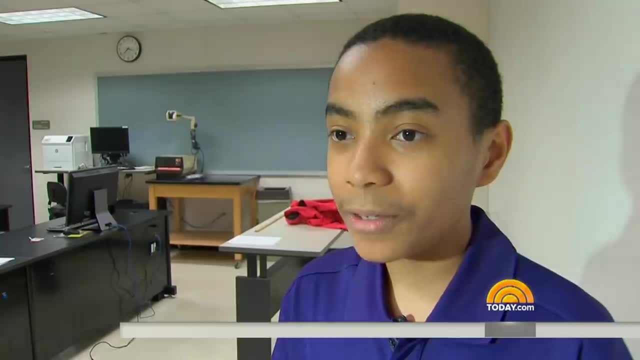 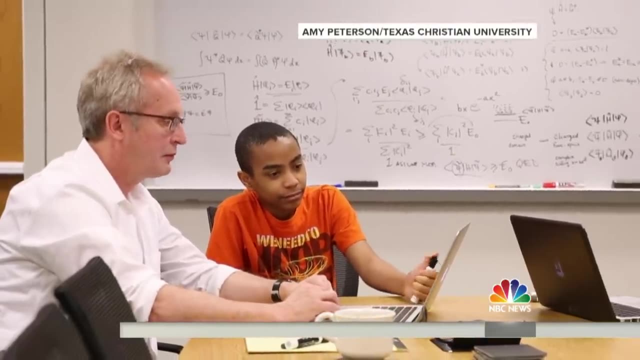 I still have friends, my age, I have a puppy, I have all of those things that you would normally have, but it's just academically different. In the fall, Carson will return to TCU for graduate school and eventually his PhD. 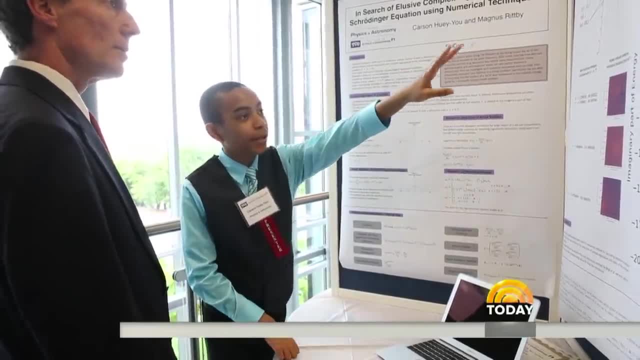 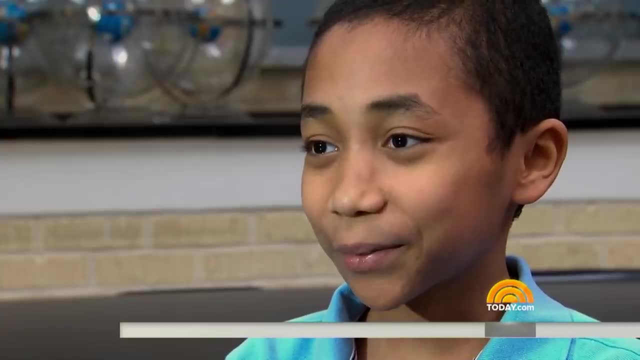 But this time he won't be the only one. He'll be the only member of the family on campus. His brother, Cannon, just 11 years old, will be a freshman When I come to TCU. I'm going to major in astrophysics and engineering. 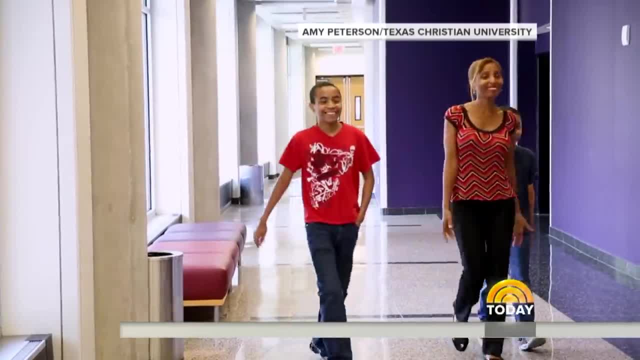 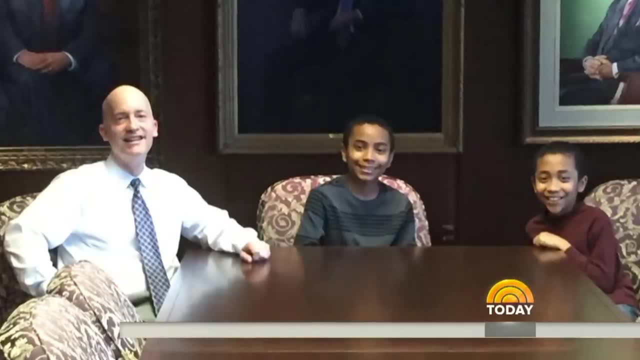 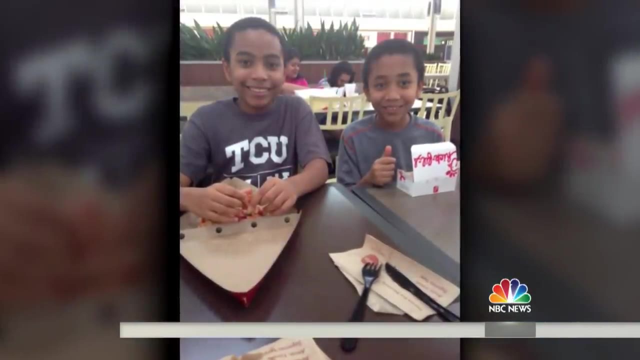 Claretta, the proud mom of the two youngest TCU students, ever says there is no magic parenting formula, just a love of learning. I was blessed that God gave me such wonderful little boys and they love to learn For Today. Jacob Rascone. NBC News Dallas. 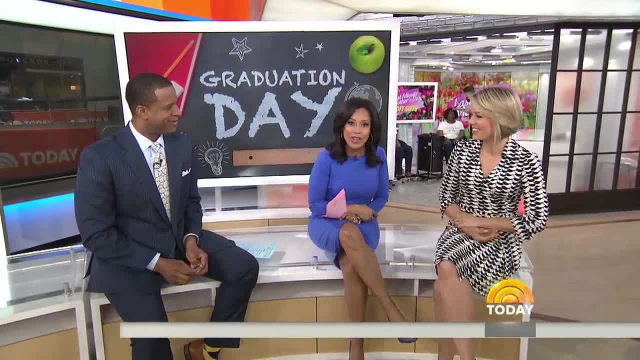 Way to go, Carson, That is impressive. What is she feeding them? Tell me the secrets. She says there's no magic pill, but I mean She's doing something. Yeah, All right, I'll find out and I'll tweet it. 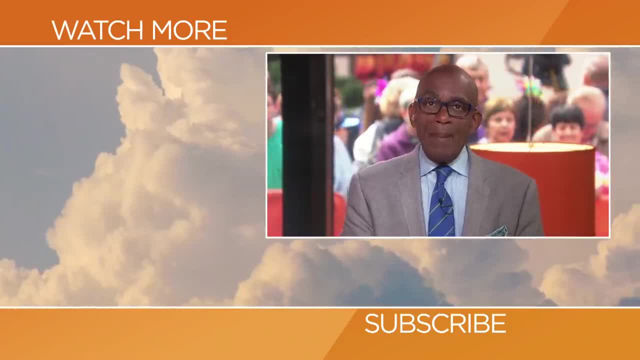 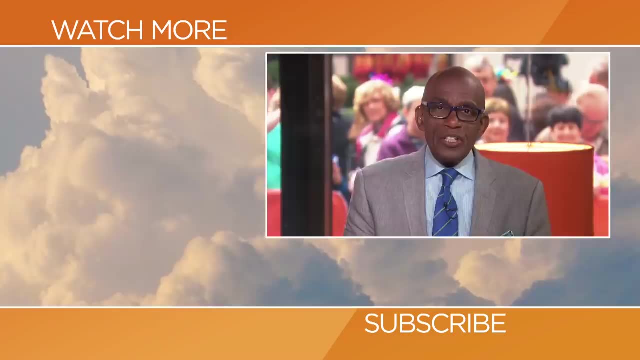 Hello Today fans. Thanks for checking out our YouTube channel. Subscribe by clicking that button down there and click on any of the videos over here to watch the latest interviews, show highlights and digital exclusives.